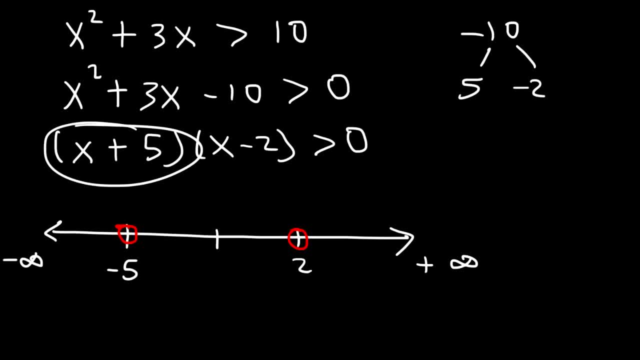 Now, 3 plus 5 is positive And 3 minus 2 is also positive. When you multiply two positive numbers together, you're going to get a positive result. Now let's pick a number between negative 5 and 2.. Let's try 0.. 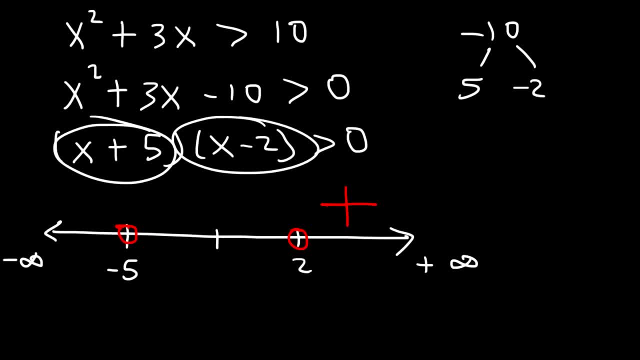 0 plus 5 is a positive number. 0 minus 2 is negative. A positive times a negative number will give us a negative number, So it's negative in this region. Now let's try negative 6. So negative 6 plus 5 is negative. 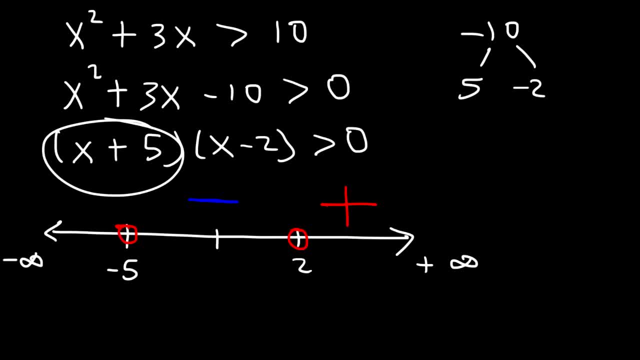 Negative: 6 minus 2 is negative. When you multiply two negative numbers, it will give you a positive number. So because it's greater than 0 and not less than 0, we want the part where x plus 5 times x minus 2 is positive. 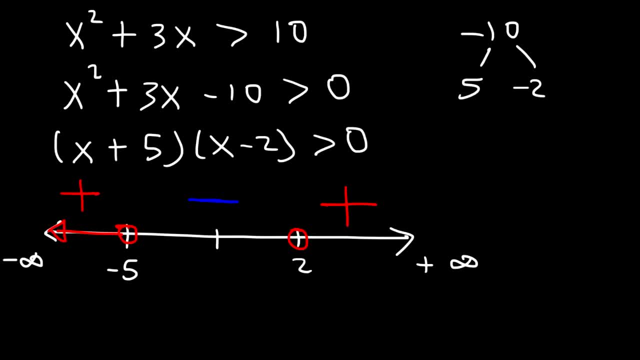 So we want this region on the left and the region on the right. So to express the answer using interval notation, it's going to be from negative infinity to negative 5, not including negative 5, union 2 to infinity. Now if you wish to express your answer as an inequality, you could say that x is greater than 2, that corresponds to this part, or x is less than negative 5, which corresponds to that part. 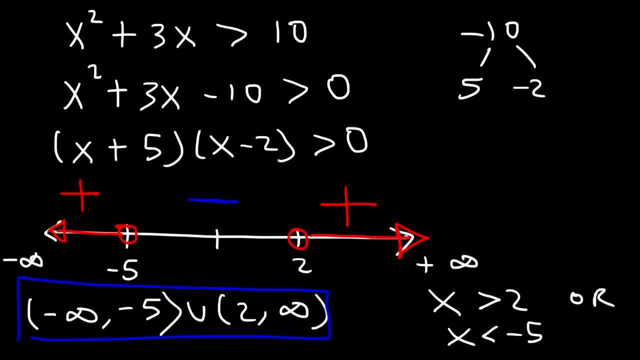 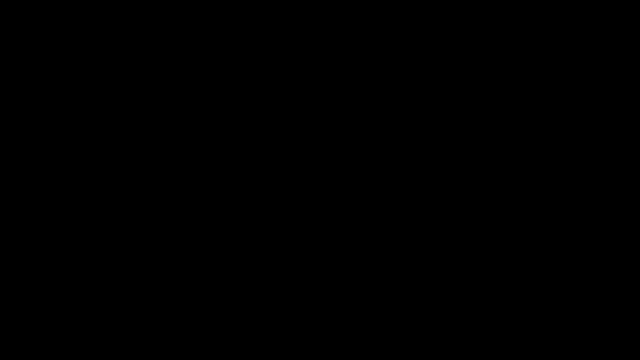 So you can describe your answer using interval notation Or using inequalities. So that's it for this problem. Let's try another example: x cubed minus x. Now let's say it's less than or equal to 3x squared minus 3.. 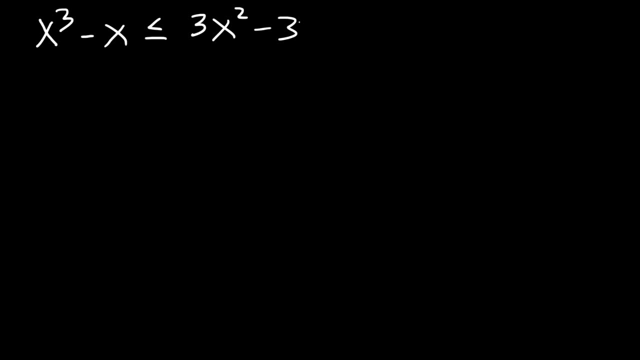 So go ahead and solve this particular polynomial inequality. So what I'm going to do is I'm going to take everything from the right side and move it to the left side And make sure you write it in steps. I'm going to write it in standard order or standard form. 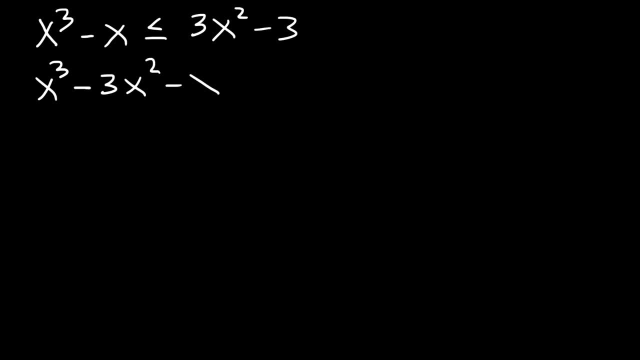 So it's going to be x cubed minus 3x squared minus x plus 3. And that's less than or equal to 0.. Now we need to factor by grouping. So let's take out the greatest common factor in the first two terms. 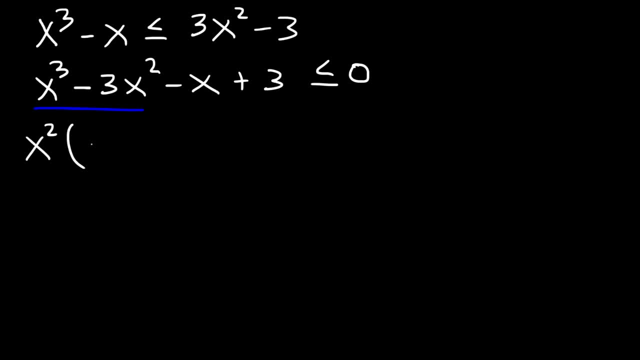 Which is going to be x squared. And so x cubed divided by x squared is x Negative. 3x squared divided by x squared is negative 3.. Now, in the last two terms, Let's take out a negative 1.. So then this is going to be x minus 3.. 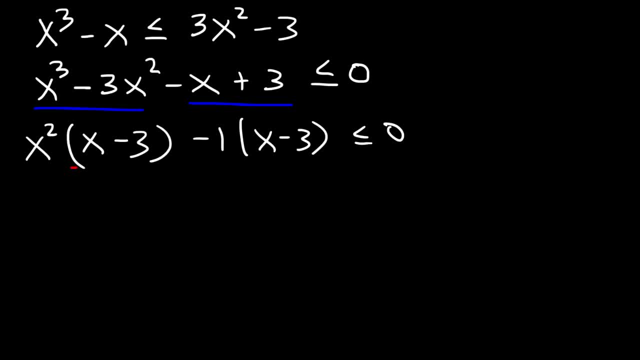 Now we can also factor the GCF. at this step We can take out x minus 3.. So if we take out x minus 3 from the first term, We're going to have x squared left over, And if we take it out from the second term, 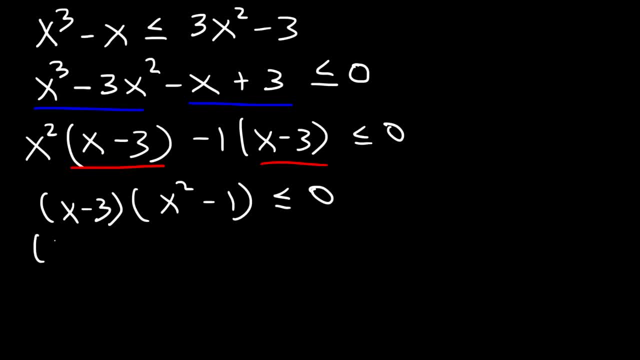 We're going to get negative 1.. Now we can factor x squared minus 1.. Using the difference of perfect squares, It's going to be x plus 1 times x minus 1.. So now let's create the number line. So there's three points of interest. 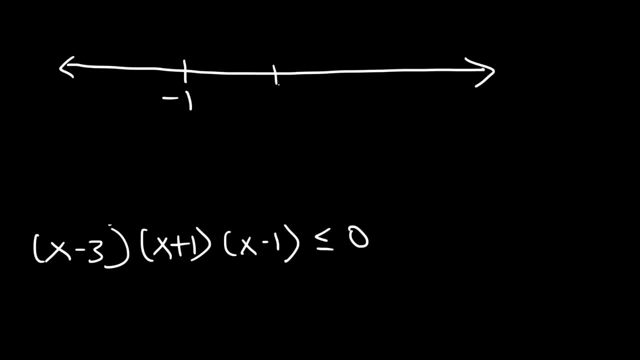 So we have negative 1,, 1, and 3.. And then, to the right, we have positive infinity And negative infinity on the left. Now Notice that it's less than or equal to 0.. Because of the underline, It's going to include these three points. 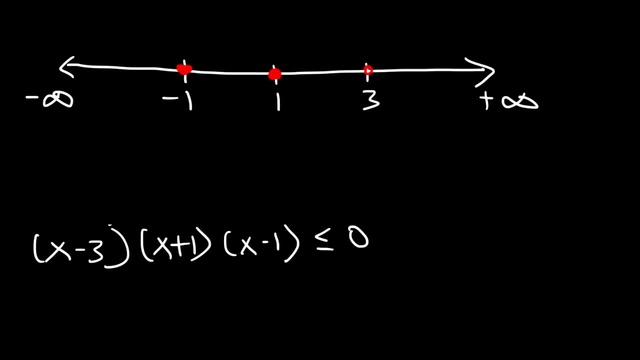 Negative: 1,, 1, and 3.. So I'm going to use a closed circle As opposed to an open circle this time. So now We need to make sure that it's less than 0 or negative, So we don't want the regions where it's positive. 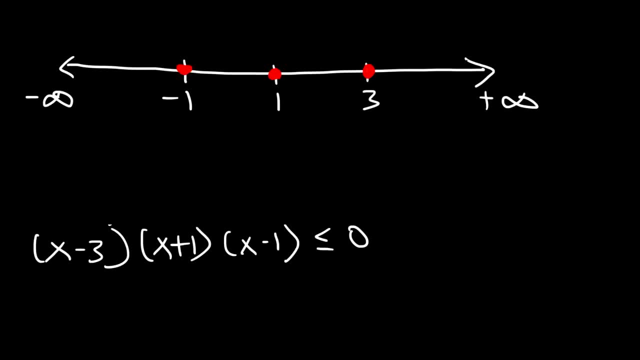 Let's test the signs. So let's start with 4.. That's between 3 and infinity. So 4 minus 3 is positive. 4 plus 1 is positive. 4 minus 1 is positive. So if we multiply three positive numbers, 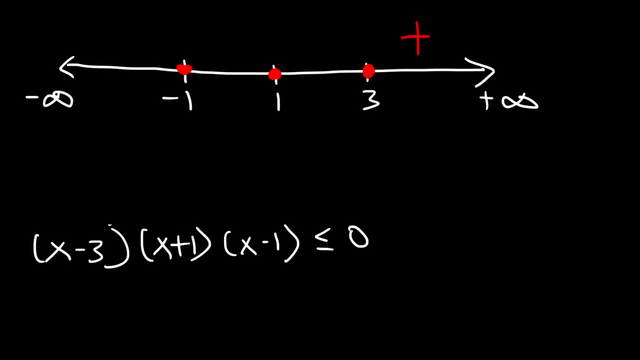 That will give us a positive result. Now let's pick a number between 1 and 3. So let's try 2.. So 2 minus 3 is negative. 2 plus 1 is positive. 2 minus 1 is positive. 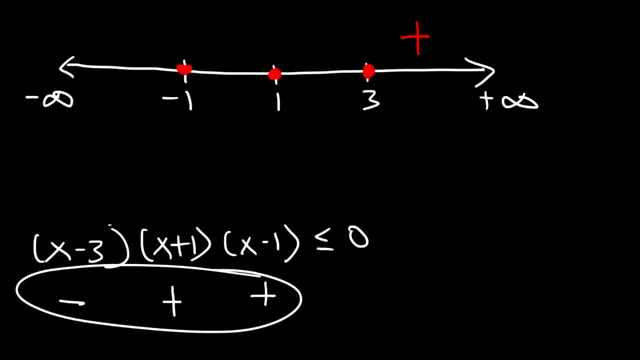 So these three signs, When multiplied together, will give us a negative number And the signs will alternate Because the multiplicities of each 0 is 1. So the next one should be positive. So let's pick a number between negative 1 and 1.. 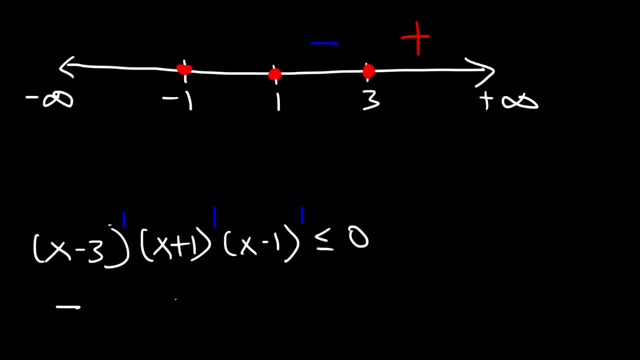 Let's try 0.. 0 minus 3 is negative, 0 plus 1 is positive, 0 minus 1 is negative. Two negative numbers will make a positive result And the last one should be negative. So if we try negative 2.. 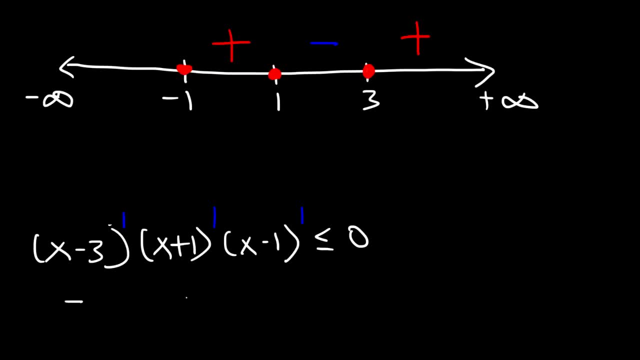 Negative. 2 minus 3 is negative. Negative. 2 plus 1 is negative. Negative. 2 minus 1 is negative. The net result is negative. Now we want the part that's negative. So we want this region And also the region between these two parts. 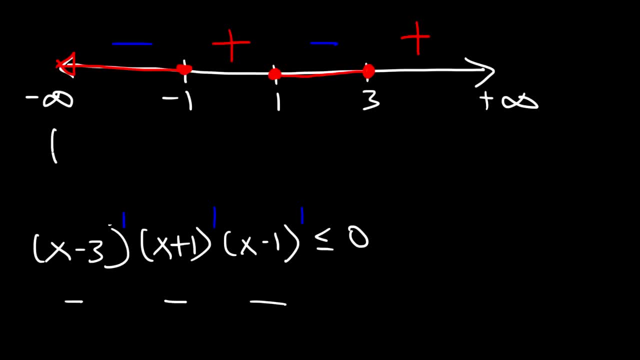 So the answer? So the answer is going to be from negative infinity to negative 1.. But including negative 1.. So we need to use brackets instead of parentheses, And then from 1 to 3.. So that's the answer, using interval notation. 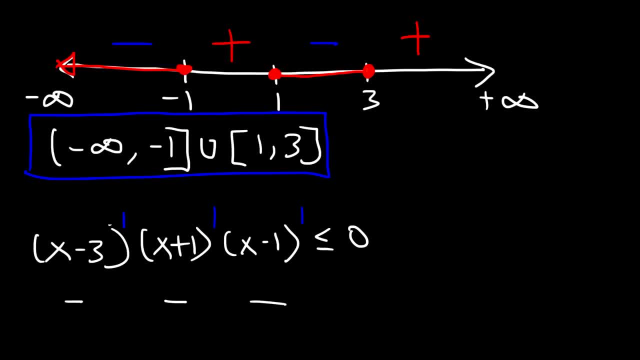 Now what's the answer? using inequalities. So for the first part, We can say that x is less than or equal to negative 1. So that covers this region. And then, for the second part, We can say that x is less than or equal to 3.. 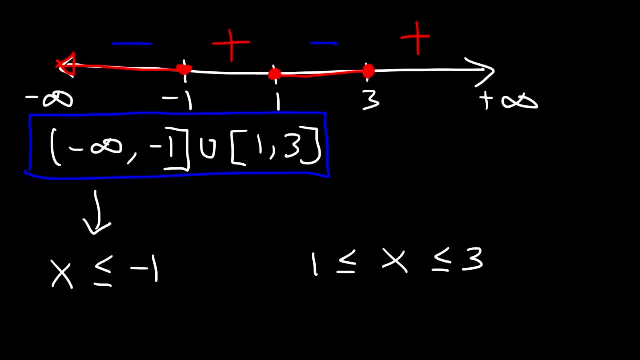 But greater than or equal to 1.. So this inequality covers this region. So let me write an OR statement. So that's the solution using inequalities. Let's work on one more problem. Let's say that x, cubed minus 2x squared, is greater than or equal to 5x minus 6.. 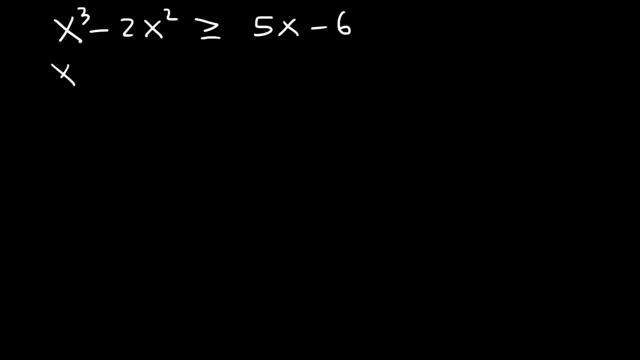 Go ahead and try that. So, just like before, Let's move everything to the left side And then let's factor. So we can't factor by grouping, So we need to use the rational zero theorem to list the possible rational zeros. So factors of 6 are 1,, 2,, 3, and 6.. 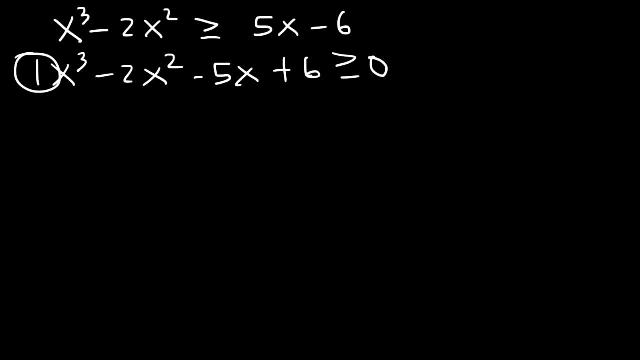 And factors of the leading coefficient are just 1.. So let's plug in numbers to see which one is going to give us 0. Then we can use synthetic division to get the other zeros. So let's start with 1.. 1 to the third minus 2 times 1 squared minus 5 times 1 plus 6.. 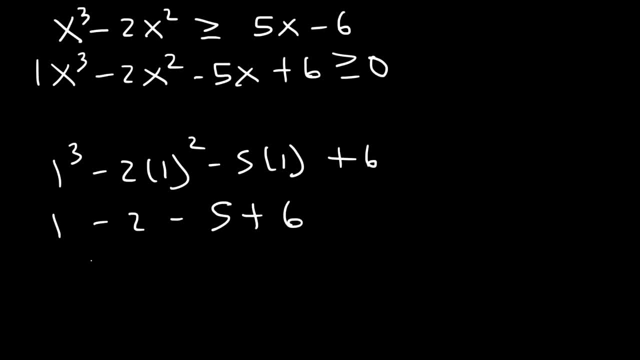 This is 1 minus 2 minus 5 plus 6. 1 minus 2 is negative 1. Negative 1 minus 5 is negative 6. If you add that to 6, you get 0. So one of the solutions to this problem. 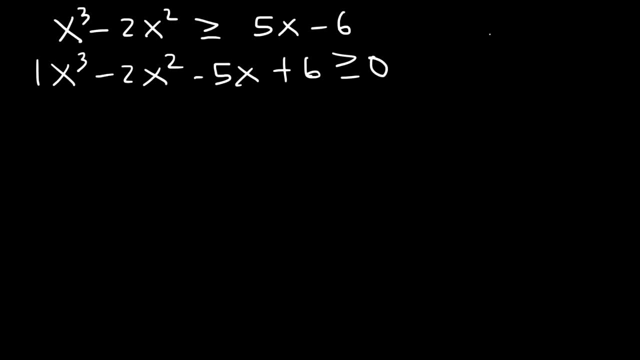 One of the points of interest is: x is equal to 1.. Now let's use synthetic division, So it's going to be 1, negative 2, negative 5, and 6.. So if we bring down the 1.. 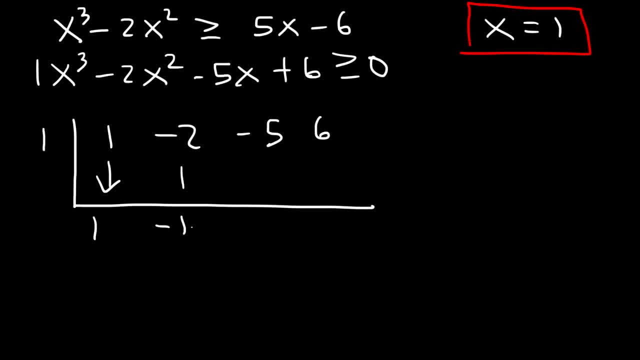 1 times 1 is 1.. Negative 2 plus 1 is negative 1.. Negative 5 plus negative 1 is negative 6. And so it's going to be 1 degree less than that. So it's 1x squared minus x minus 6.. 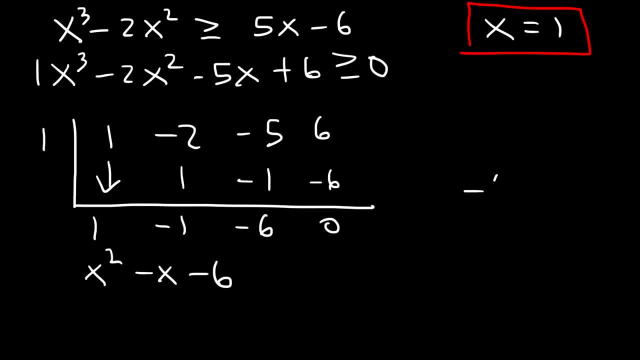 And now let's factor this expression: Two numbers that multiply to 6 but add to negative 1 is going to be negative 3 and 2.. So we can factor this as x minus 3 times x plus 2.. And x equals 1 is related to this factor. 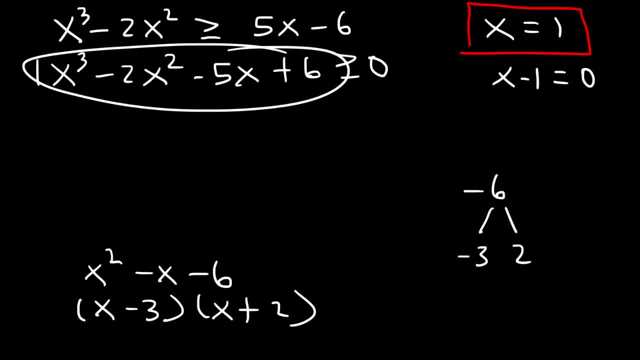 So to completely factor this expression, It's going to be x minus 1 times x plus 2 times x minus 3.. So the other points of interest are negative 2 and 3.. So x equals negative 2 and positive 3.. 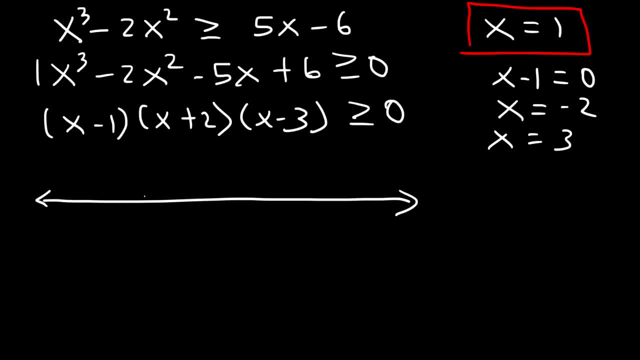 Now let's make a number line, So the lowest x value that we have is negative 2. And then we have 1 and then 3.. Now those points are included because it can be greater than or equal to 0. So let's draw a closed circle. 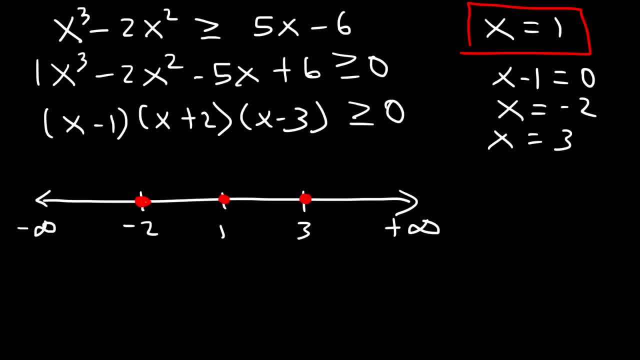 And we need to find the areas where it's positive. So let's start with a number that's greater than 3.. Let's try 4.. So 4 minus 3 is positive. 4 plus 2 is positive. 4 minus 1 is positive. 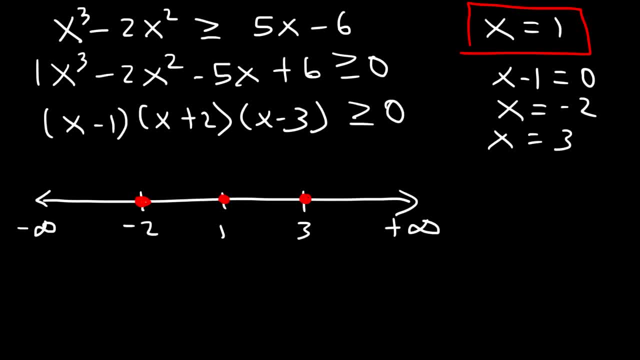 So we need to find the areas where it's positive. Let's try: 4.. 4 minus 3 is negative. 3. 5 minus 1 is positive. 5 plus 2 is negative. 5 plus 3 is positive. 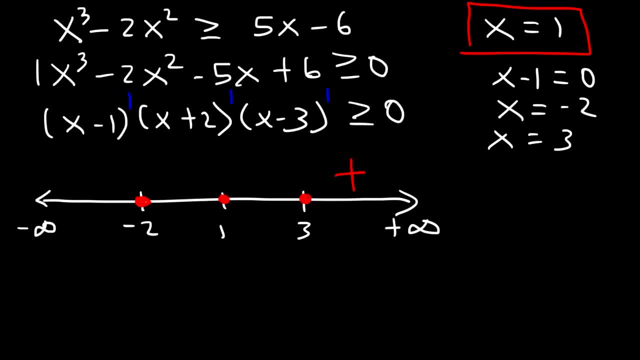 5 plus 2 is positive. So we can now go back to our Friedmann equation. Now, where did we leave off this time? We left off with a right answer, So right answer is 0.. So we have x plus 1.. 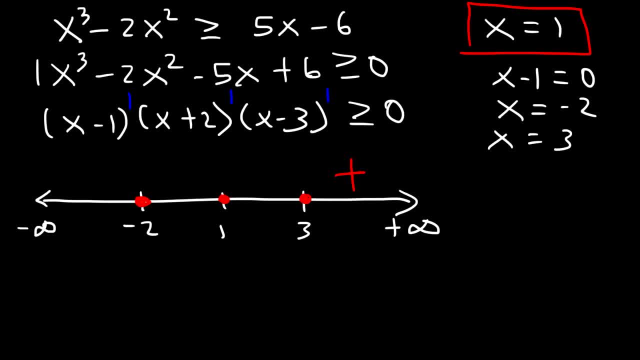 And our right answer is 0.. So there's no right answer there. There's no right answer there. So we're going to deal with the right answer And here's the right answer. OK, Right answer. One of the right answers is negative: 1 and 2.. 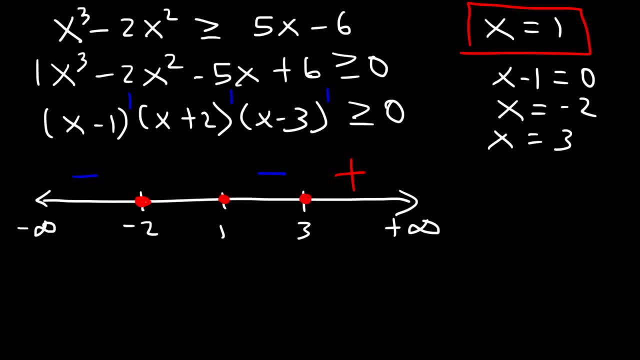 So the right answer is negative 1.. But an odd answer is negative 1.. But then the opposite is also a right answer and it's just going to alternate sign. So we only want the region where it's positive. So that's between negative 2 and 1, and between 3 and infinity. 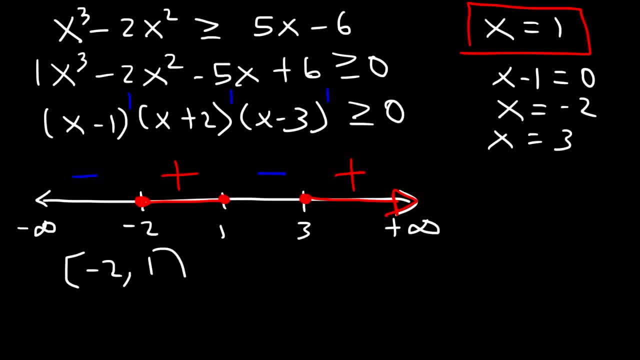 So in interval notation the answer is from negative 2 to 1,, union 3 to infinity, And as an inequality we could say that x is less than or equal to 1, and greater than or equal to negative 2, or x can be equal to or greater than 3.. 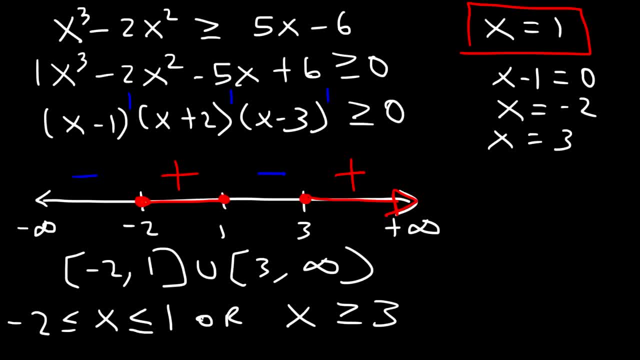 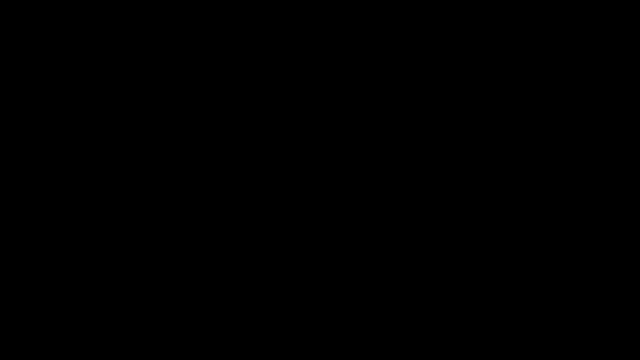 So we can write it like that And that's it. So now you know how to solve a polynomial inequality using number lines and interval notation. Thank you.